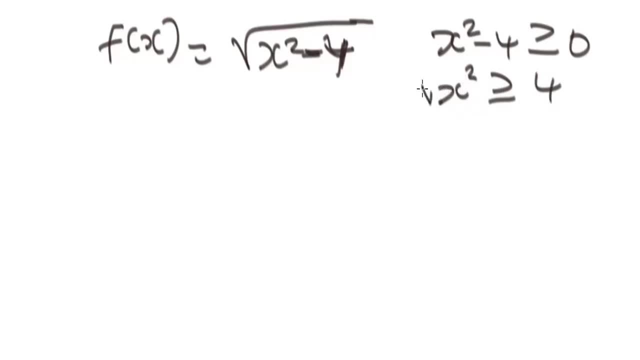 So, to make it as well, you square both sides. So x is greater than or equal to 4.. Sorry, greater than or equal to 2, square root of 4 is 2.. So that means the range of this function, y. 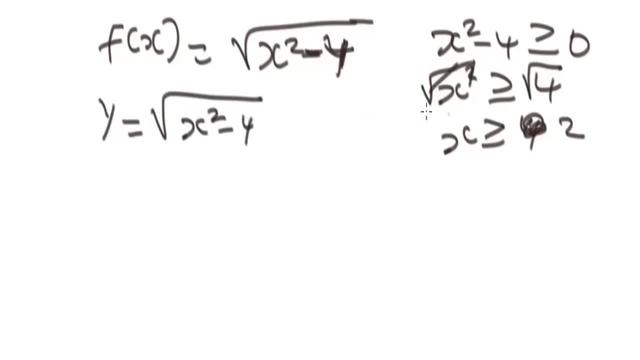 equals square root of x square minus 4, will be. when you plug in to here, it will give you 4.. 2 square is 4, 4 minus 4 is 0. So the range of this function will be all the numbers from 0 to infinity. 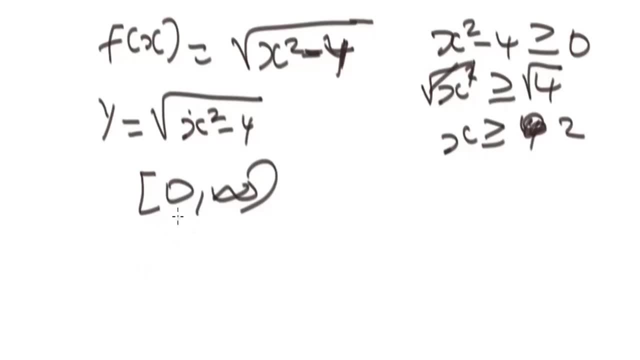 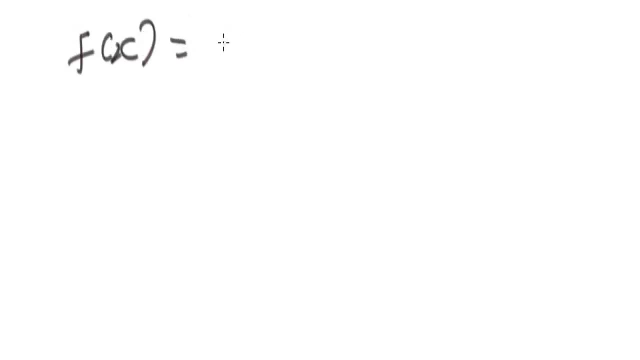 including 0.. So that will be the range of this function. So let's try this, try this answer on our problem. Okay, let's say we are given this function, We have f of x equals 1 over square root of x minus 3.. 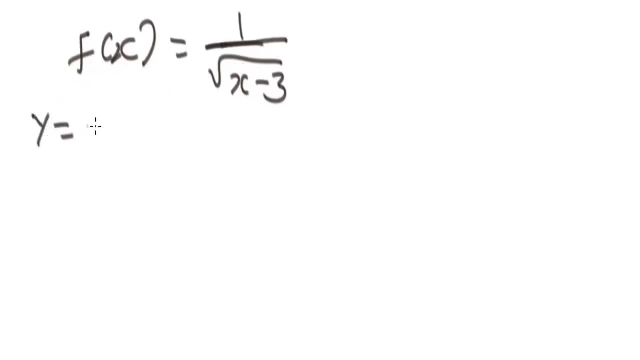 So how do you find the range of this function? Remember, f of x and minus y equals 1 over square root of x minus 3.. So first of all, you have to make x inspect x in terms of y. so if you express x in terms of y, 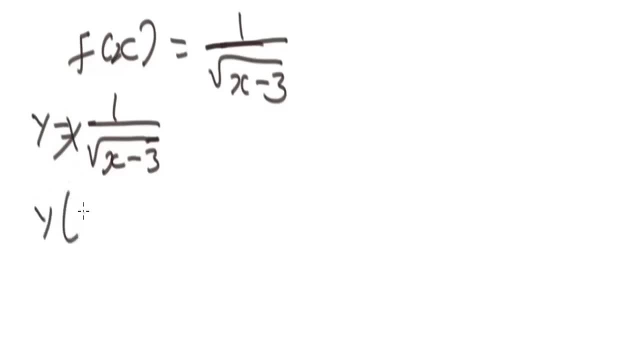 let's multiply this, so we're going to have y in brackets square root of x minus 3, okay, equals 1.. So to make this square root, you square both sides, okay. so this now cancels your way. 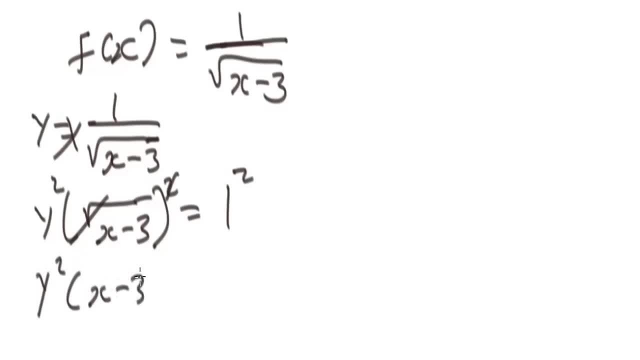 left it y square times x minus 3, equal 1. square root of x minus 3 equals 1.. So we're going to simplify this. then we're going to have y square x- okay, minus 3y square equals 1.. 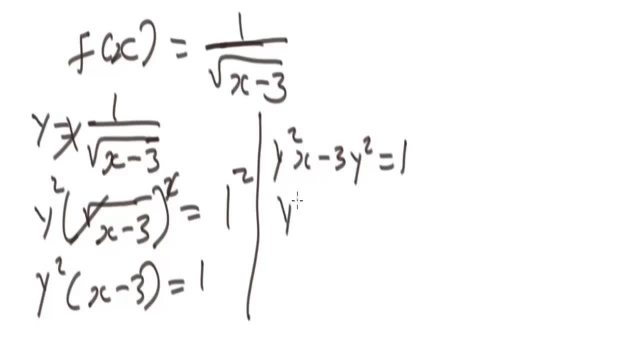 So remember, we want to make x the same formula. We're going to have first y square, x equals 1 plus when this goes over 3y square. so you make a derivative from the divided both sides by y square. So the x equals 1 plus 3y square over y square.